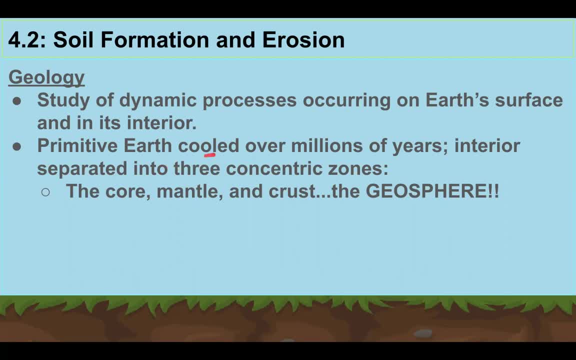 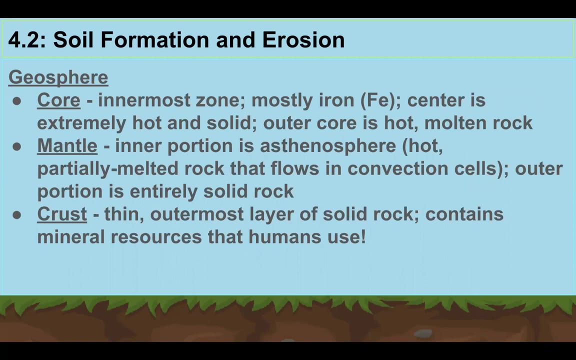 that the heat, some of it, which was lost over this period of millions of years. there's still quite a bit of heat at the center of the Earth. So the core, mantle and the crust. we'll talk a little bit about the core and the mantle and then we're going to continue talking about the crust through the rest of this section. 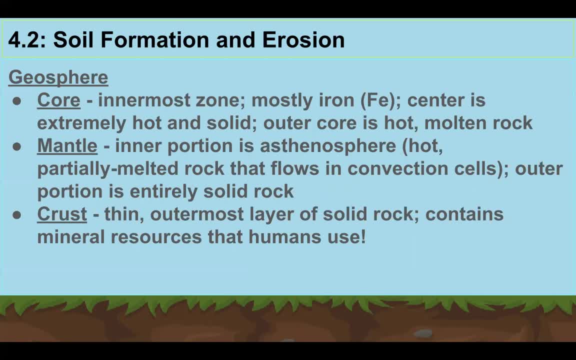 So the core is the innermost zone, So it is the center of the geosphere. It is made out of mostly iron and it is very hot, So there is quite a bit of heat. There is quite a bit of energy there in the center of the Earth. The inner core is solid. The outer core is actually molten. 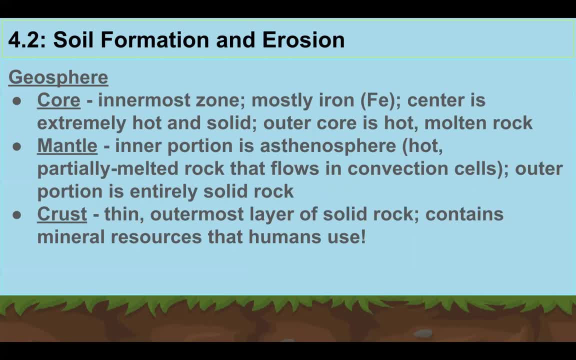 Okay, The mantle is probably the thickest part of the geosphere. The inner portion is the asthenosphere, where it is made up of partially melted rock. It flows into the atmosphere And convection currents are- remember. it's going to be very hot near the core And the hot molten rock is going to flow up towards the surface, where it will cool down and then flow a little bit off to the side before going back towards the core. 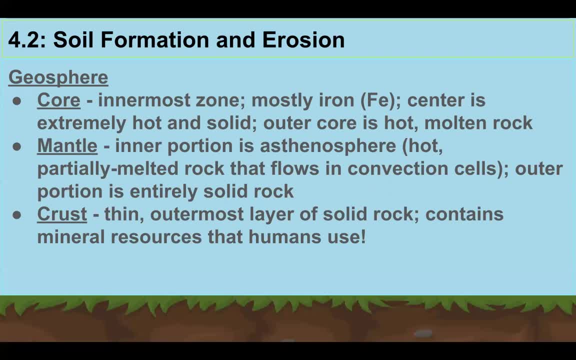 That would be a convection cell. The outer portion of the mantle is entirely solid rock, where it will be part of the tectonic plates along with the crust, And then the crust is the outermost layer of solid rock. It is cool. It is not very hot like the mantle or the core are, And the crust contains all the mineral resources that we, as humans, use. 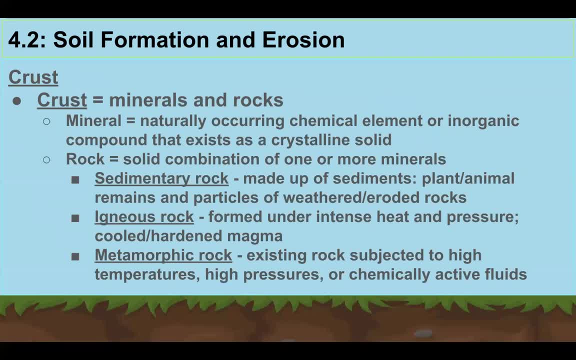 Okay, so a mineral is defined as a naturally occurring chemical element or inorganic compound that exists as a crystalline solid. So we'll be talking about You know something like, maybe something like a crystal. You know something like, maybe something like a crystal? 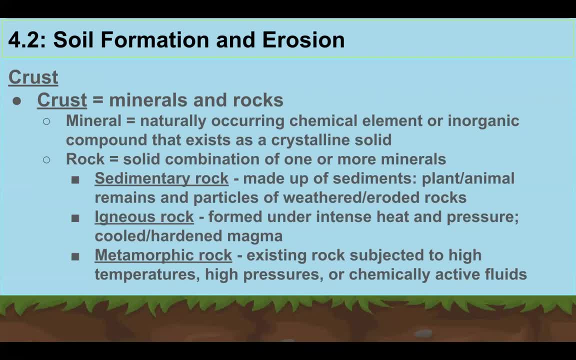 You know something like, maybe something like a crystal, Maybe silicone, Silicon dioxide, Like you know, a quartz. There there are many minerals that we utilize, that we get from the geosphere in a crust, So there are three different types of rocks and 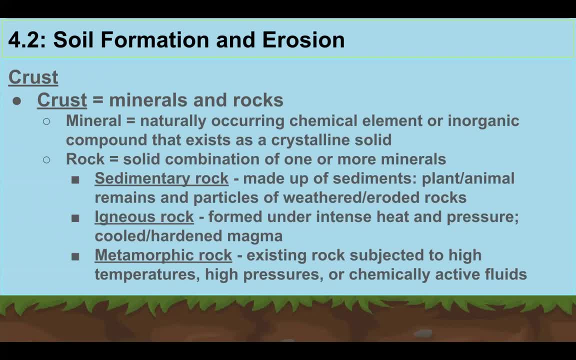 so sedimentary, igneous and metamorphic rocks. A sedimentary rock is A rock that is less durable, is made up of many sediments right that have come together to form the rock, and plant. animal rains can become part of sedimentary rock too, and okay, so it's really just a a big conglomerate of all. 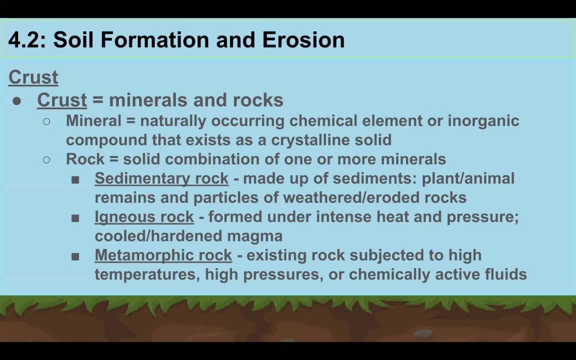 of these sediments together, an igneous rock is formed from magma, so it is magma that is cooled and hardened and so it started as as a liquid magma that had been cold and hardened. metamorphic rock is existing rock, so it could be your sedimentary or igneous rocks, but is an existing. 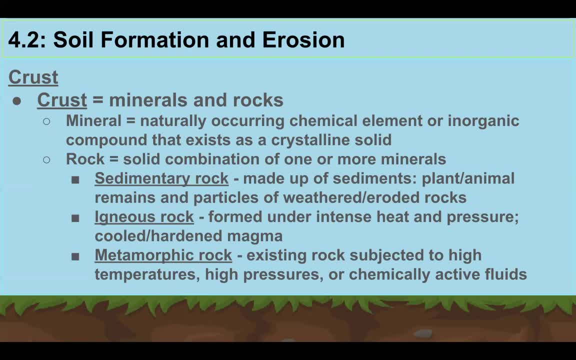 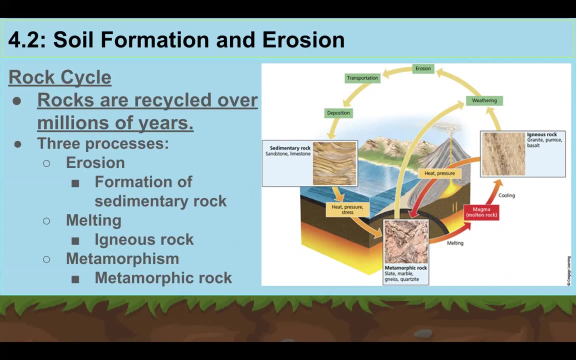 rock that has been subjected to high temperatures or high pressures, or even chemically active fluids, so it causes the metamorphic rock to change in some way. okay, so rocks. there's even a rock cycle, and they're- they're recycled over millions of years. so there are a few processes at play, so erosion is the one that we're most familiar with that. 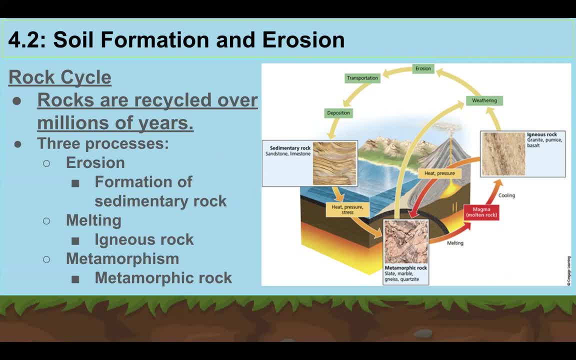 occurs at the crust surface, erosion will result in the formation of sedimentary rock. when rock is melted, it can then become igneous rock once it does cool down and harden. and metamorphism is just uh. remember the the high amounts of heat or pressure or uh chemical substances that can cause the rock to change uh in form. 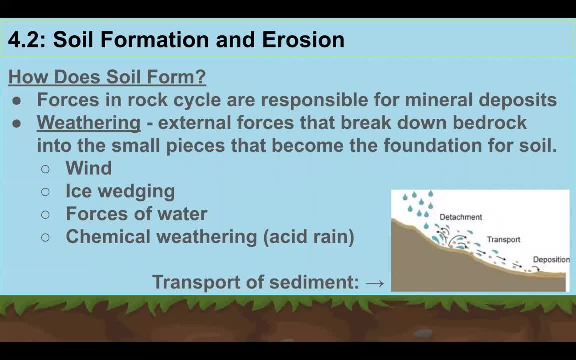 so there are a few cycles that are going to be important in the formation of soil. okay, so what we just talked about is the formation of rock. soil is kind of going to be the breakdown rocks. okay, Weathering is probably one of the most important processes here. This. 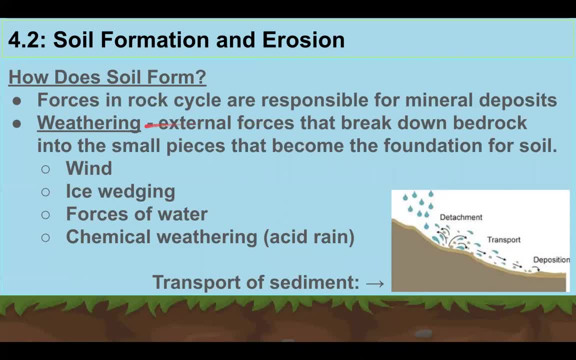 is just where an external force, such as wind, or perhaps the breaking apart by water or ice wedging, which is when water gets in between pores in a rock and then cools down and freezes and expands and breaks apart the rock. in that way We can. 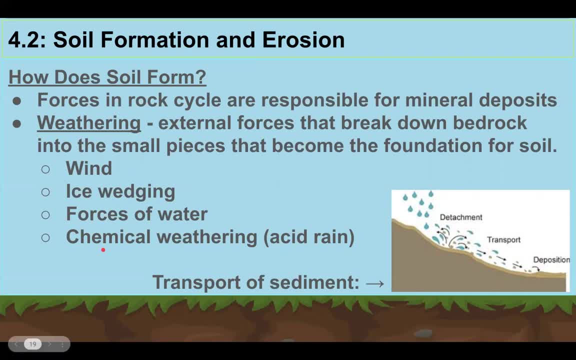 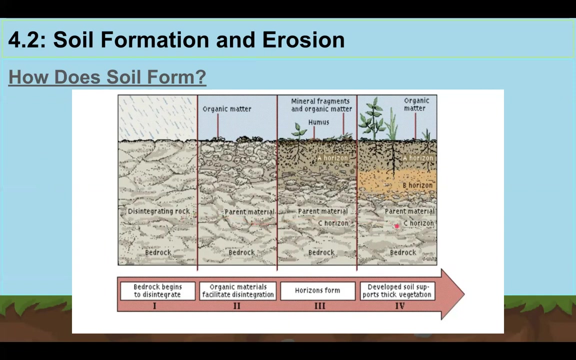 be talking about chemical weathering like acid rain. so the reaction of the acid rain with a substance in the rock- Think of something like limestone? okay, But sediment is going to get transported through runoff right by. it gets carried off by water, All right. so just over time, rock is going to break down from these. 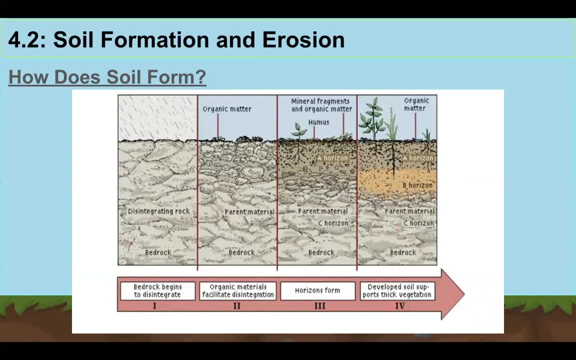 various processes- okay, these weathering processes, And as the rock begins to break down, right, a contributor could be certain organisms, like lichens, that contribute to the breakdown of the rock by releasing chemicals that will cause chemical weathering. All right, but those are going to die, And as the living 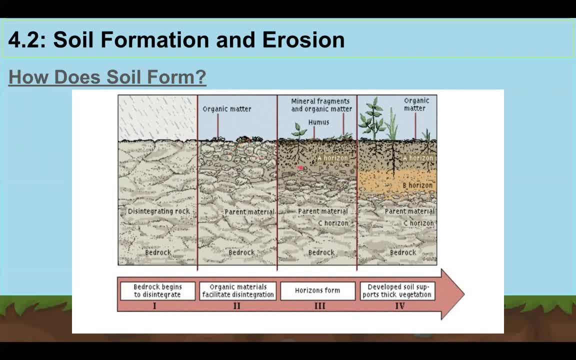 organisms die, their remains will become part of the soil, So providing a little bit of nutrients there, And eventually we're going to get a mix of the rock which is heavily broken down now, where we have much tinier sediment as well as organic matter, the humus, And eventually 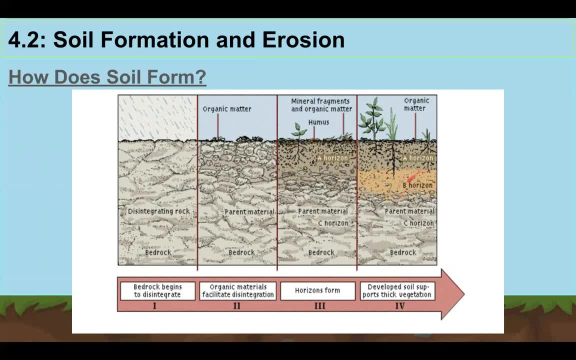 it's actually going to stratify, where we'll actually have several layers of distinct parts of the soil. all right, Still have the bedrock down here, but instead of being completely rock now it's going to become a lot of that has broken down the soil that we have here. 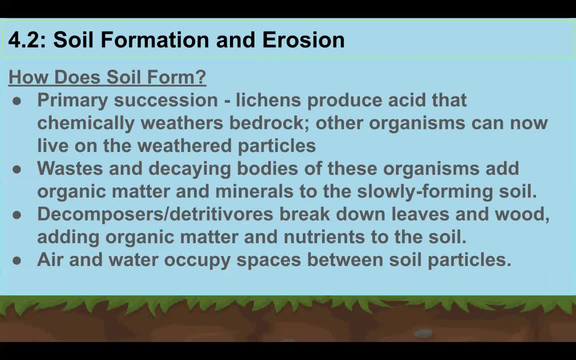 Okay, so primary succession uses this process right, the weathering processes that will break down the bedrock and start to form the soil. Don't forget that organisms, as they die, their bodies are going to get broken down and the nutrients that they 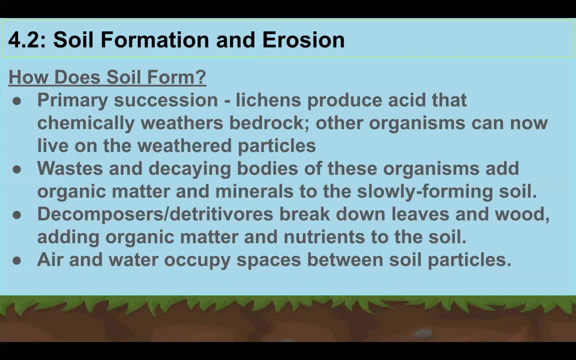 had in their organic matter are going to become part of the soil. okay, So organic matter is a very important part of soils. Decomposers and detritophores are going to break down these dead organic matter, or perhaps waste, or even leaves that have been shed by trees. 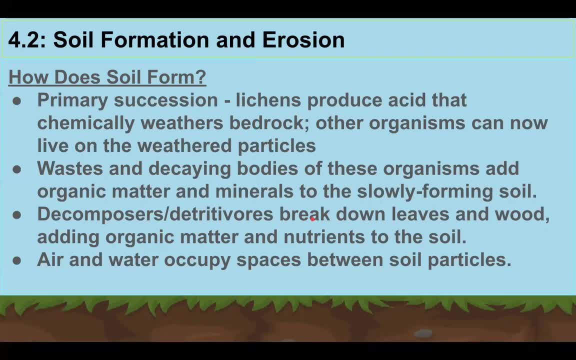 and that will contribute to the nutrient levels in the soil And probably the most important part of soil. okay, it's not just the sediment, it's not just all of the nutrients, but air and water also need to be there, because those two things are going to. 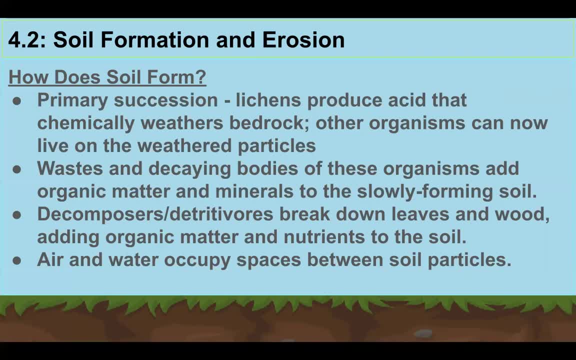 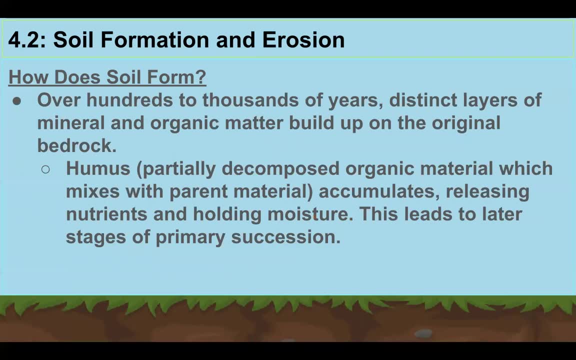 support the growth of plants in water, in soil. excuse me, All right, so this is a process that takes quite a long time, can be hundreds of years, maybe thousands of years, depending on the, the, the amount of, like rainfall or wind or something like that- but the, the minerals and the organic. 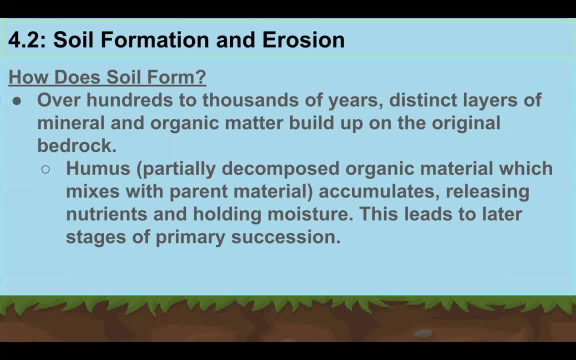 matter are going to build up over time and humus, which is the partially decomposed organic matter that is going to accumulate again. It is incorporated into the soil and the organic matter as it continues getting broken down will release nutrients in the soil. 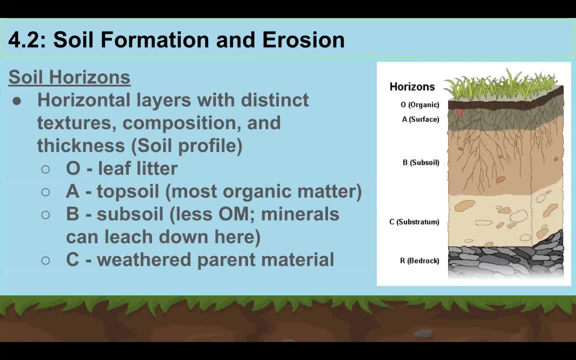 Okay, So here are the layers. here We have the O layer, which is pretty thin. That's mostly just the organic matter, like leaf, litter and stuff like that. The A surface, which has a bunch of the sediment plus a lot of organic matter. B has less organic matter. 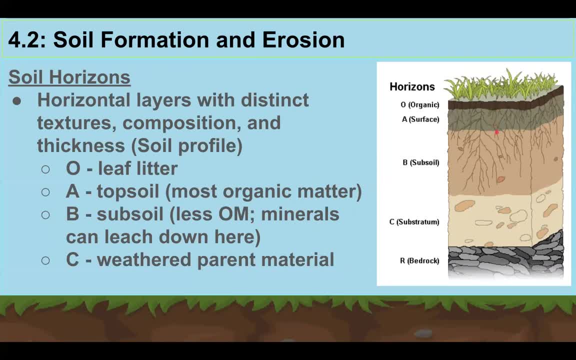 Minerals might leach down here, meaning that they, like, will kind of fall off, Get carried by water Down to B. C is the weathered parent material, So it's not the solid rock like we have down here, but it is this rock as it continues getting broken down, Okay, before it really is incorporated as part of the soil. So there's gonna be a lot of rock down here in the C. 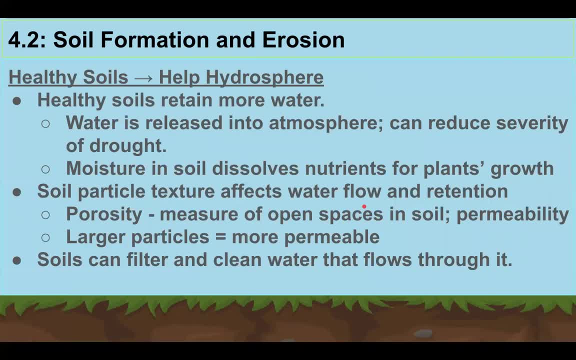 layer or horizon. All right. so healthy soils are going to be ones that can retain water- All right. water needs to be able to flow through, Yes, but water also needs to be retained. So a good mix of the different particles in the soil will help to not just let water flow through, but also will let the water. 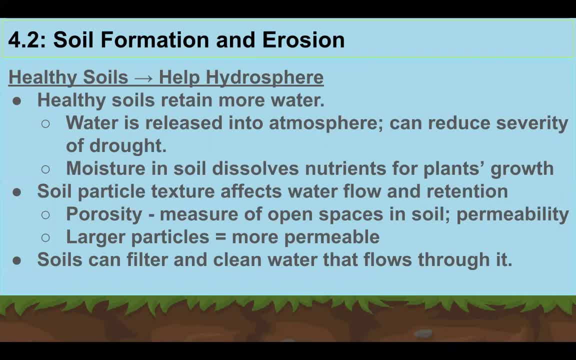 you know, will help to hold the water there too. So soils retain water, and that water can evaporate and go into the atmosphere, So that can be helpful in some weather conditions. The moisture in the soil helps to dissolve nutrients that plants will only be able to get. 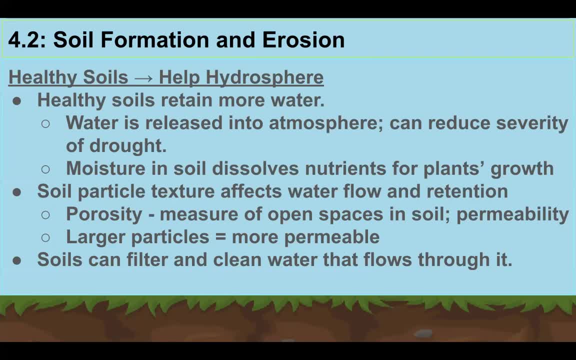 from water. So that is another important characteristic of soil and why water is important there. The particle texture is going to affect the water flow in the retention that we were just talking about. So there are really three main categories for the particle texture that we'll be talking about shortly. so the larger 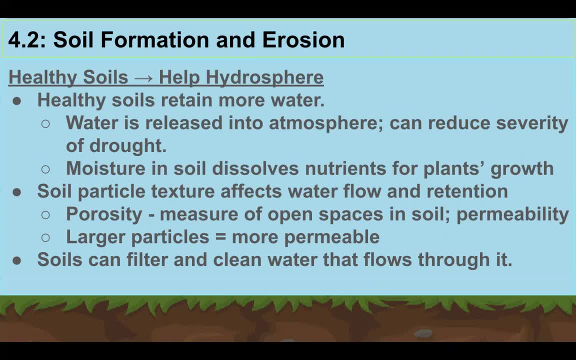 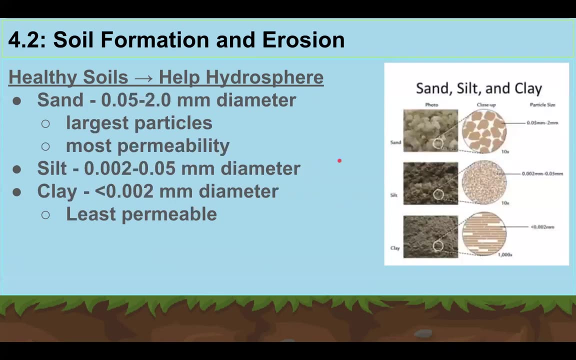 particles are more permeable and allow for more porosity or more spaces between them. okay, and another rather important part of soil is that, as the water is flowing through, it filters and cleans the water. okay, so our different size particles here: sand, silt and clay, so sand is the largest. 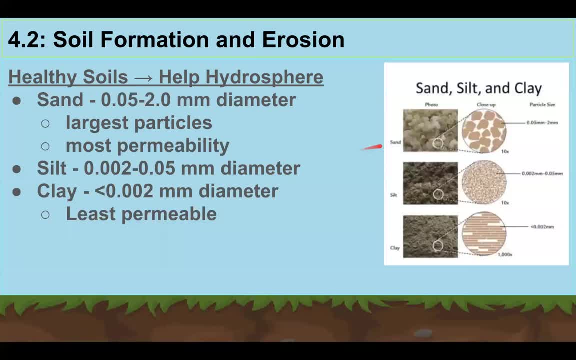 it is the most permeable. so the largest gaps in between these particles: silt is, in between, much smaller than the sand particles, but also still bigger than the clay. all right, so small, less permeability because, as you can see, there's less space in between each. 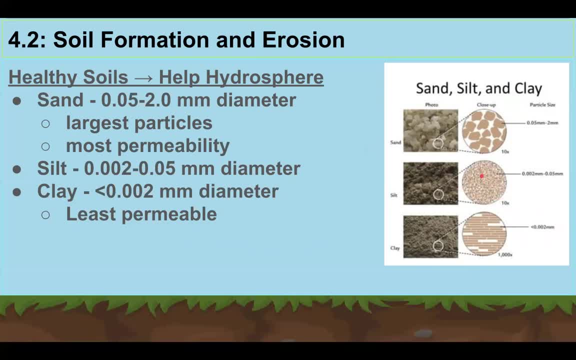 of these, just because they're smaller, and clay is smaller, so it's a little bit more permeable. clay is the least permeable, it is the smallest, and so water will not really be able to flow through here, but an important part of any soil is going to be our clay. that would help to retain. 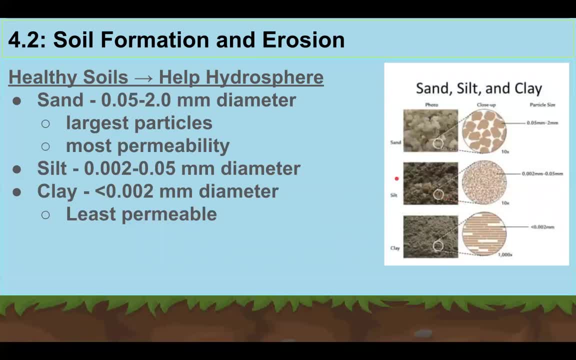 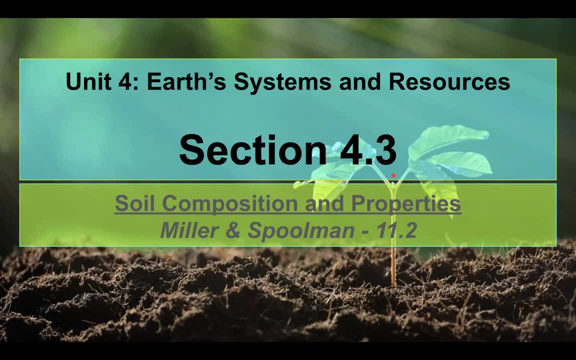 the water. okay, we just can't have too much of the clay. there is such thing as having too much of a good thing. all right, so that's going to bring us to our next section, 4.3, so let's get right into it and look at the composition of soil. all right, so think about what are the 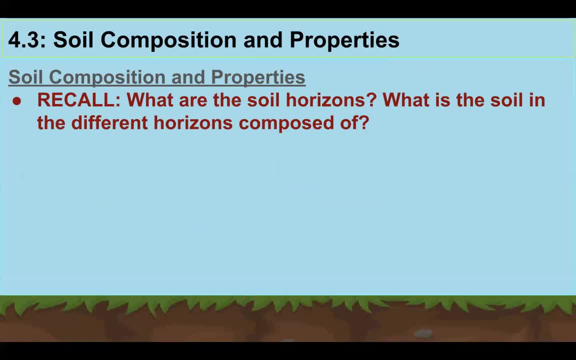 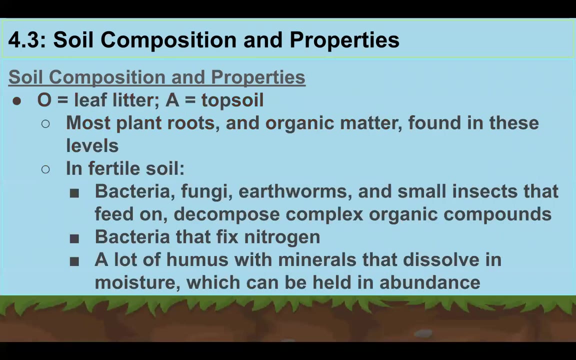 soil horizons again. so remember the a horizon, the b horizon and the c horizon, and then, at the very top, the o horizon. so think about what those are, what they were composed of, and let's um talk about the net. so towards the top, right at the top, you'll have o, and then right underneath that is a. 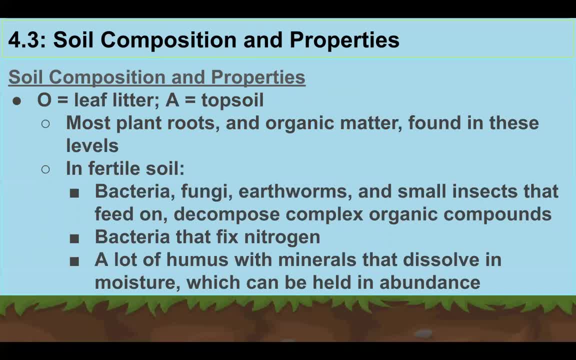 so this is where most of the organic matter and soil is going to be found, because it is the closest to the top. that's where most plant roots are going to be. that's where the leaf litter and the other decaying organic matter is going to be. 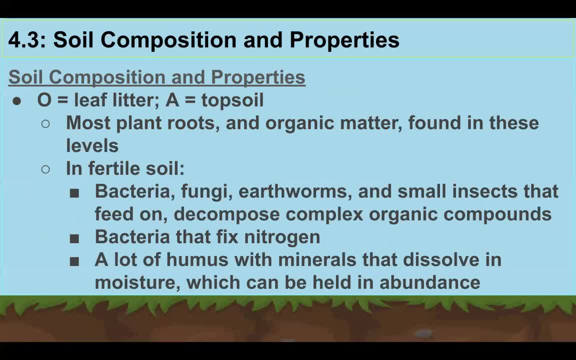 so, naturally, that a is going to be where organic matter is going to be primarily found, but o is going to be where the leaf litter is, so that's going to be on top of our soil. so in fertile soil we're going to have some organisms that help to decompose and aerate. 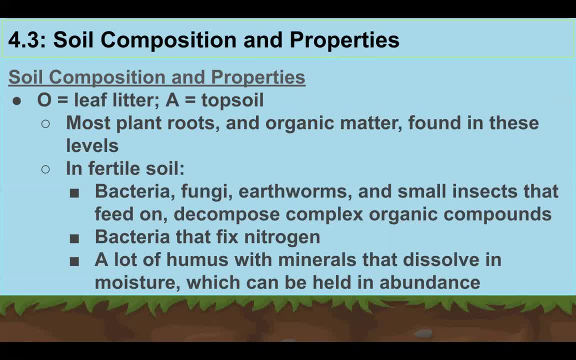 the soil. um, there will be bacteria that can help to fix nitrogen. so remember, plants can't use n2 from the air. bacteria helps by converting that nitrogen into usable forms for our plants, and there should also be a lot of humus, which will contain minerals and nutrients that need. 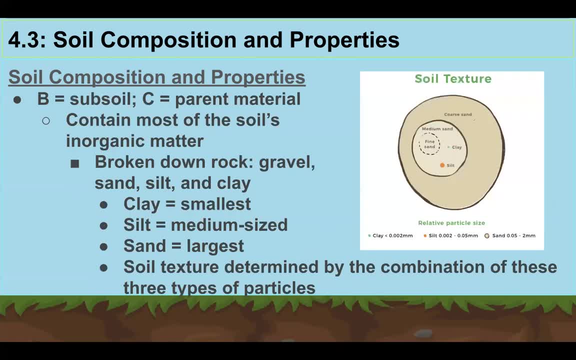 to be used by plants. okay, underneath that we have the subsoil and the parent material. so b and c. this is where most of the organic matter of the soil is going to be, because this is where a lot of the rock is either being broken down or minerals are going to be leaching down into. 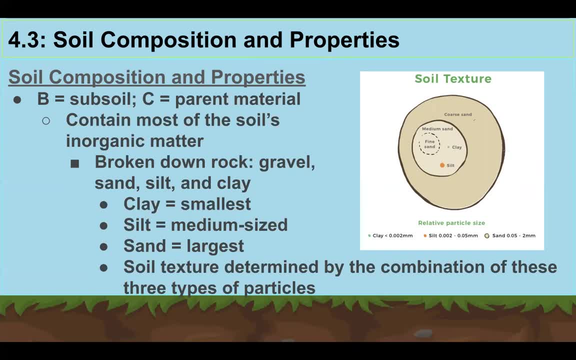 this layer from above through water. okay, so subsoil and parent material. uh, they contain the um broken down rock particles, so gravel is quite big, sand is smaller, silt is even smaller and then clay is the smallest yet. Okay, so you can take a look over here at this chart. 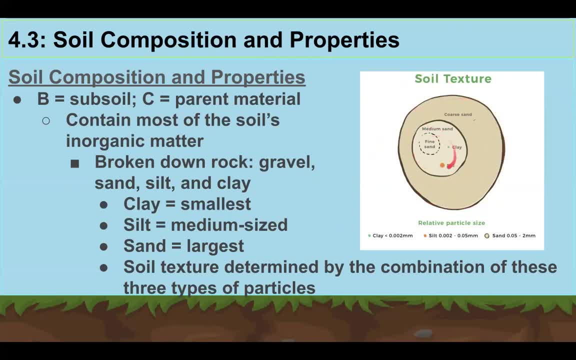 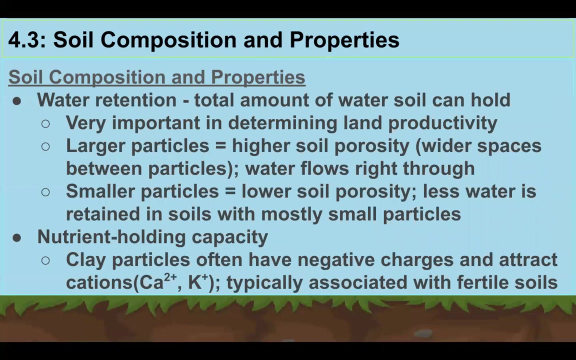 So sand is the largest particle right. there can be several classifications of sand, but even the fine sand is still much bigger than silt and even that much bigger than clay. So even clay is going to be just a small part of the silt. Okay, so the texture of the water, I'm sorry of the, of the soil, plus the. 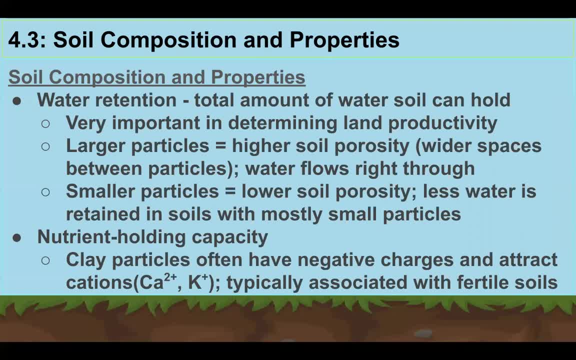 water retention of the soil is going to be dependent on how much clay, how much silt and how much sand there are there is in the soil. So remember the water retention, that's the amount of water that can be held by the soil. Land productivity is heavily dependent on that because if the soil can, 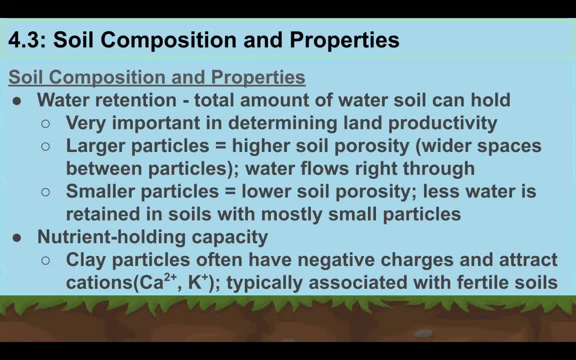 hold water, then that's good. If it can't, and that's not going to be very good for primary productivity, where plants need to get their water from the soil. Okay, so the larger particles, like the sand, have higher soil porosity, but water is not going to get held by it, so it just kind of flows right through. 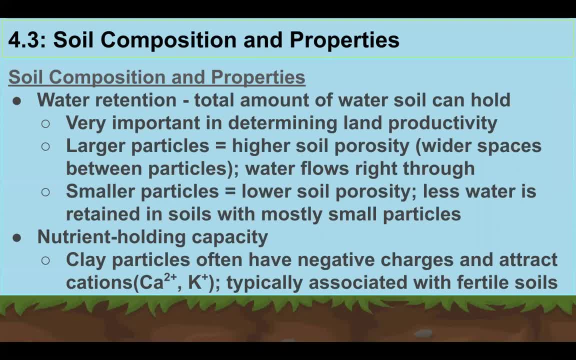 The small, the- excuse me, the smaller- particles do not have as much porosity, but they will help to retain the water, At least what can get in there. So we need a balance between these larger and smaller particles to help to retain water- All right, get it in the first place and then to retain it too. 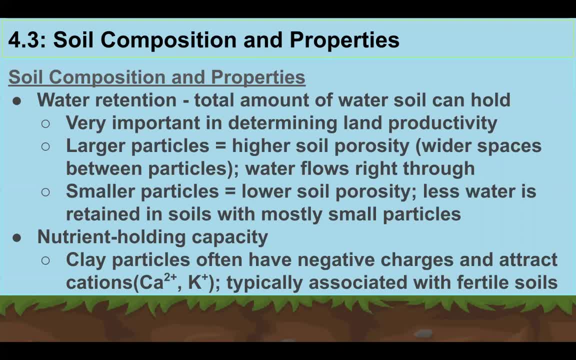 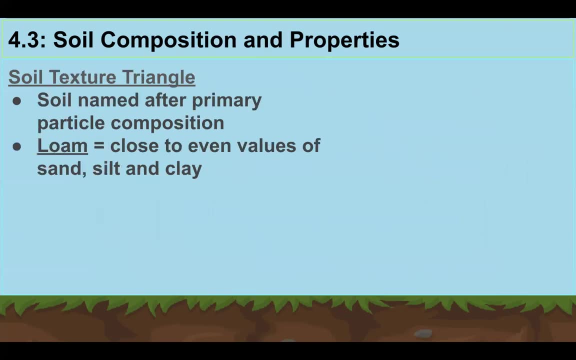 In addition to that, clay particles typically are negatively charged. They attract cations like calcium or potassium that have positive charge, So having a decent amount of clay will be good and allow soil to retain. Okay, so this is our soil texture triangle and you're going to need to be able to read this. 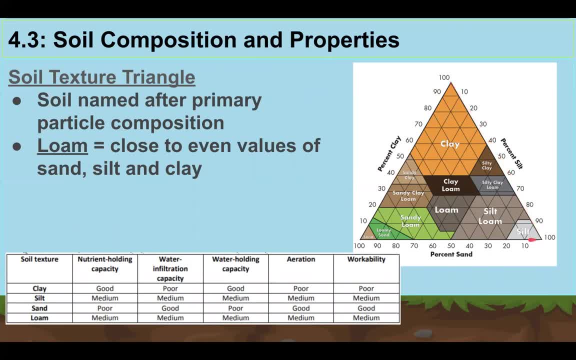 Okay. so what we are looking at here is the percentage of clay, silt and sands. Any point on this graph is going to have a certain amount of each of these particles. So if you look at this graph, you can see that this is the percentage of clay, silt and sands.